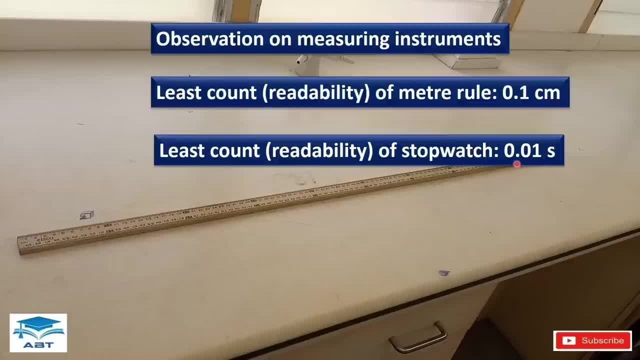 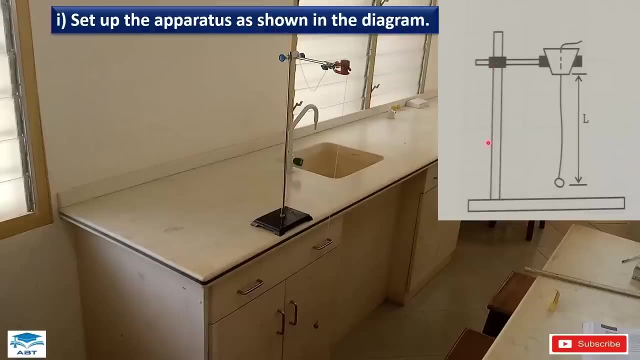 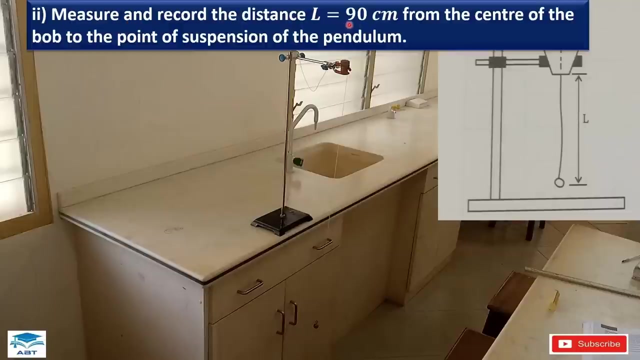 stopwatch can measure is 0.01 seconds, And also the time should be in two decimal places. Setup the apparatus as shown. Measure and record. the distance L is equal to 90 centimeters from the center of the bulb to the point of suspension. Measure and record the distance L is equal to 90 centimeters from the center of the bulb to the point of suspension. 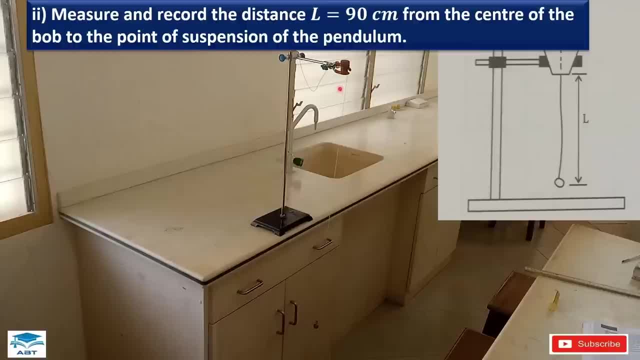 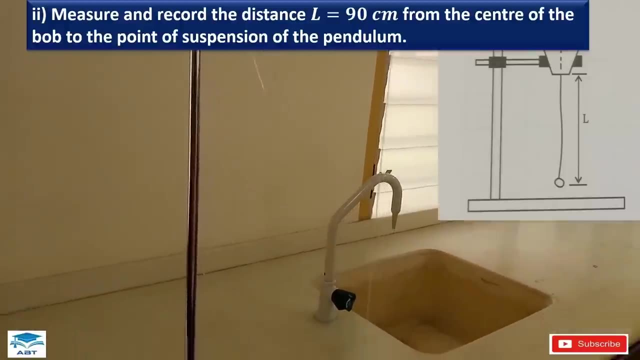 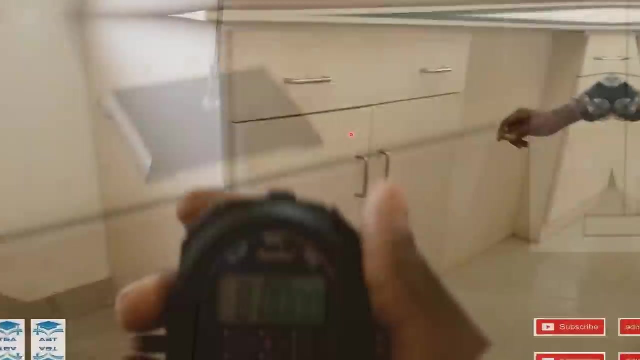 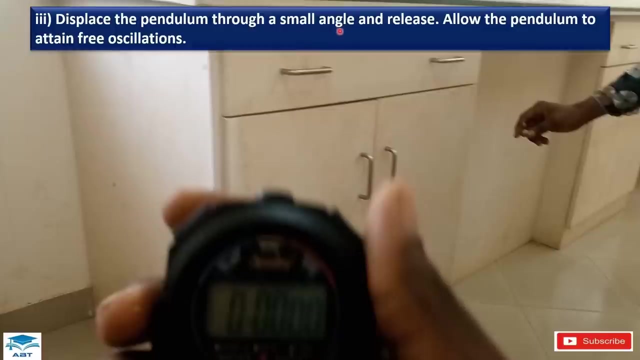 of the pendulum. so we measure a distance of 90 centimeters from the base of the split cork to the center of the pendulum bulb. we are going to displace the pendulum bulb through a small angle and release it and allow the pendulum to attain free oscillations and determine the time. 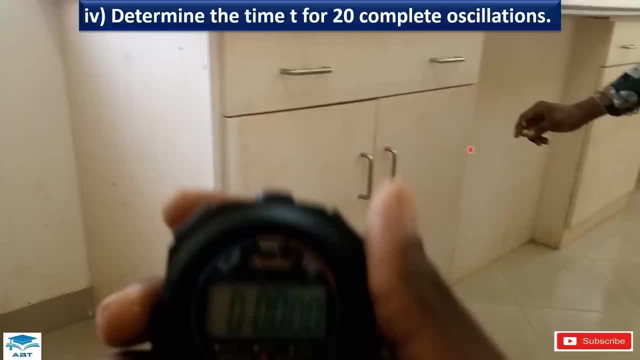 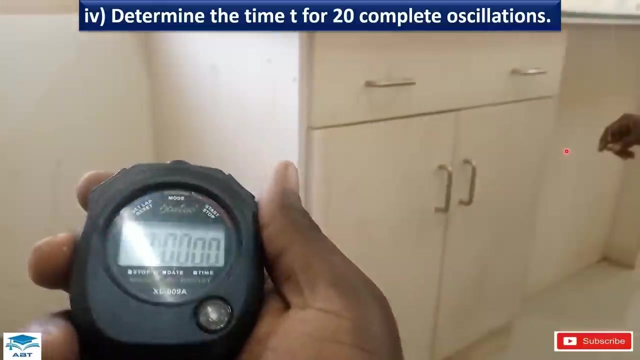 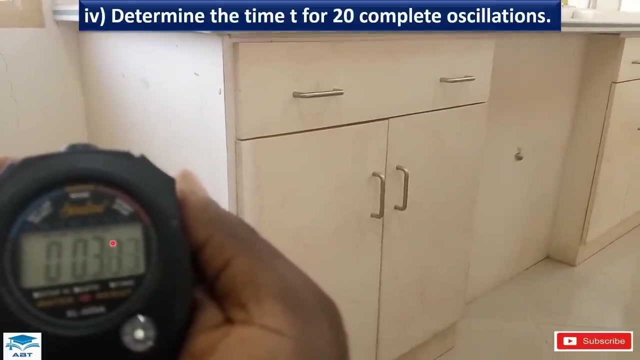 for 20 complete oscillations. when we release the bulb from this direction and it moves to this direction and comes back, it will be counted as one complete oscillation and we are going to determine the time for 20 complete oscillations. you 1,. 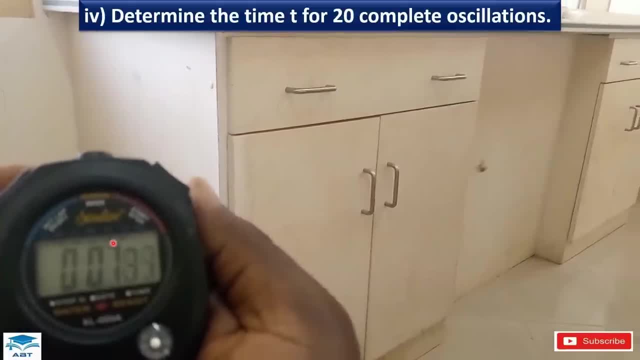 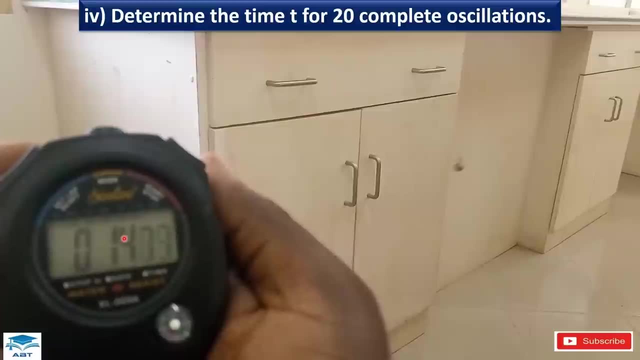 2,, 3,, 4,, 5,, 6,, 7,, 8,, 9,, 10,, 11,, 12,, 13,, 14,, 15,, 16,, 17,, 18,. 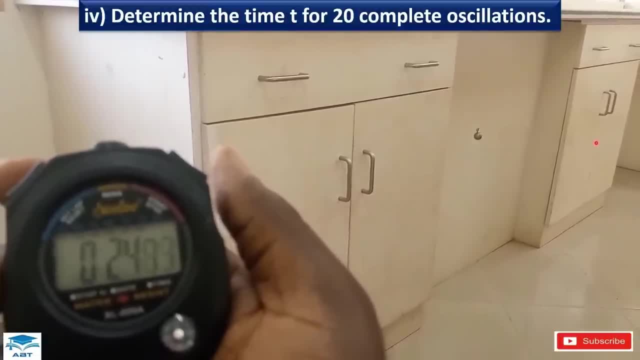 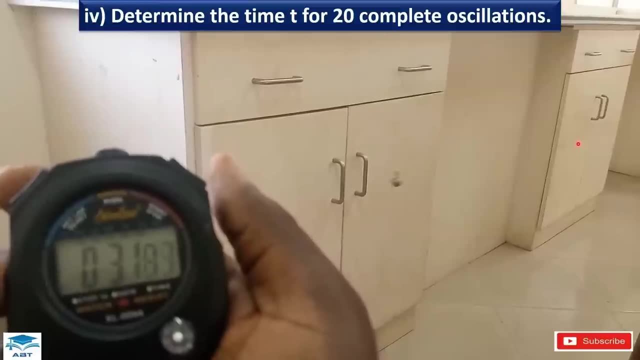 19,, 20,, 21,, 22,, 23,, 24,, 25,, 26,, 27,, 28,, 29,, 30,, 31,, 32,, 33,, 34,, 35,. 36,, 37,, 38,, 39,, 40,, 41,, 42,, 42,, 43,, 43,, 44,, 45,, 46,, 47,, 48,, 49,, 50,. 51,, 52,, 53,, 54,, 55,, 56,, 57,, 58,, 59,, 60,, 61,, 62,, 63,, 64,, 65,, 66,, 67,. 68,, 67,, 68,, 69,, 70,, 71,, 72,, 73,, 74,, 75,, 76,, 77,, 78,, 79,, 80,, 81,, 82,. 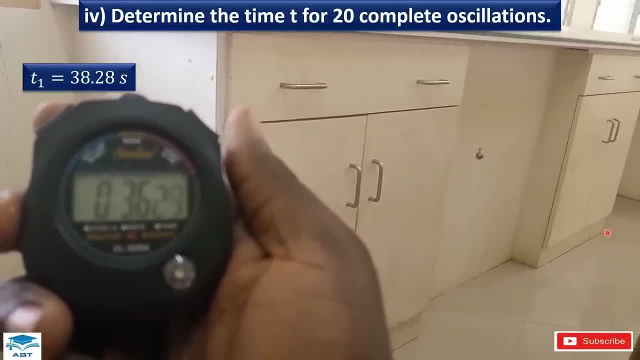 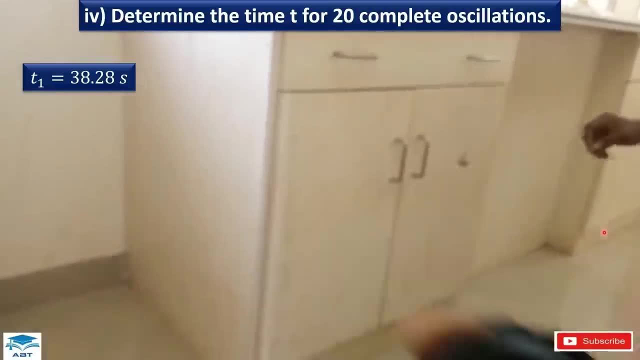 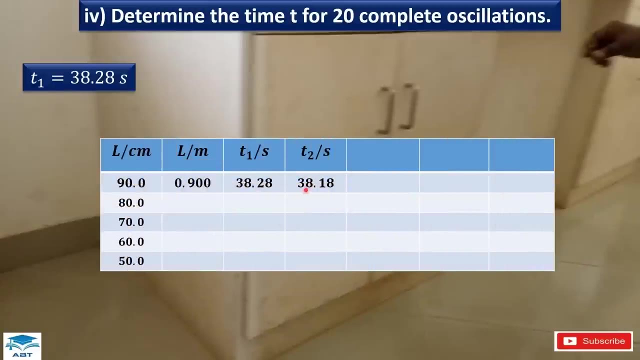 83,, 82,, 83,, 84,, 84,, 85,, 86,, 87,, 88,, 89,, 90,, 90, and 20.. So the time T2 for 20 complete oscillations is 38.18 seconds. 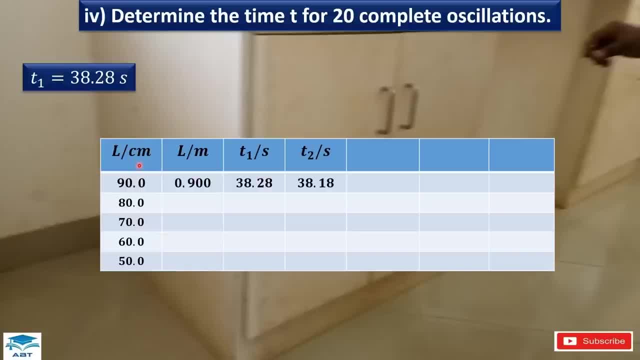 So the length of the inextensible string is 90.0 centimeters. Remember, the least count of the length of the string in the meter rule is 0.1 centimeters. That means all the values falling under the length should be in one decimal place. 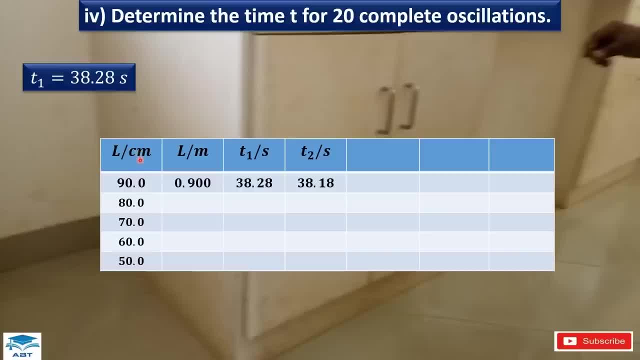 So we have 90.0 centimeters But we have to convert the length to meters, That is the SI unit of length. So 90 divided by 100 will be 0.9.. But the least count is 0.1.. 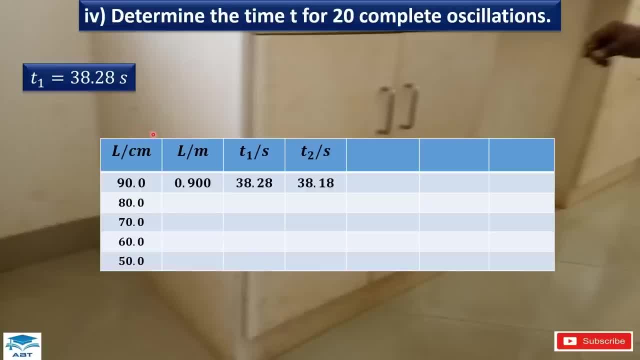 When we divide 0.1 by 100, we have 0.001.. That is three decimal places. So the length should be in three decimal places. The length in meters should be in three decimal places. This is the time one in seconds. 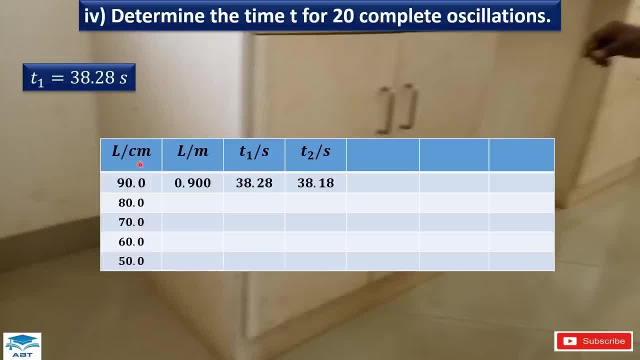 time two, also in seconds. The unit should be written here at the top once and it shouldn't be repeated with the values. Then we find the mean of the two times. That will be 38.28 plus 38.18 divided by two. 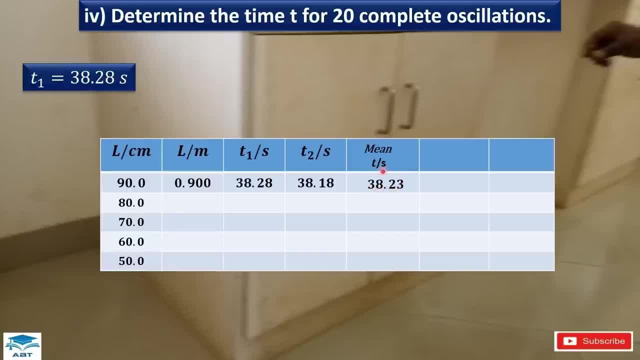 That is 38.23 seconds. Then we determine the period of oscillations and evaluate the period squared. We have the period in seconds. The period is the time for one complete oscillation And the mean time is the time for 20 complete oscillations. 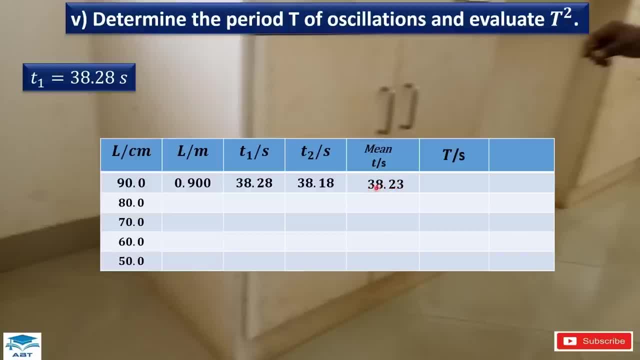 So when we divide the mean time, or the average time by 20, we have the period. So 38.23 divided by 20 will give us 1.91.. And we square the period And the unit will be second squared. 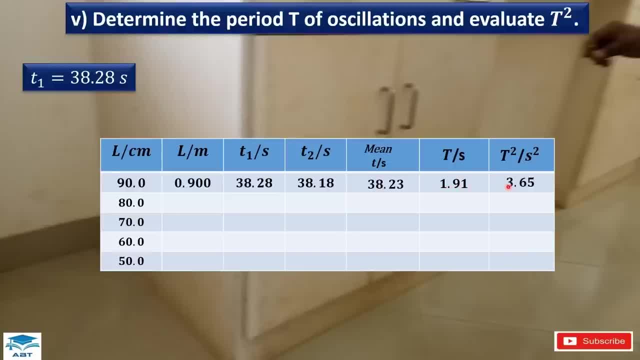 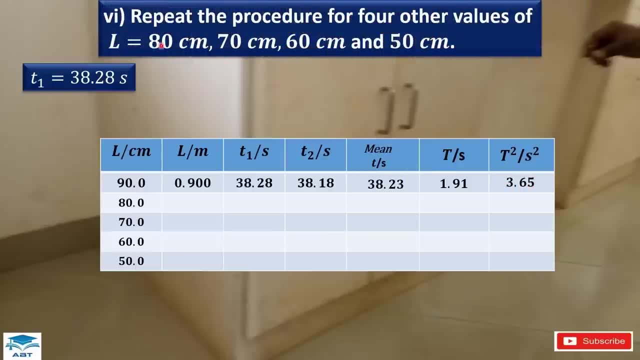 So 1.91 squared is 3.65.. Then we repeat the procedure for four other values. of length is equal to 80 centimeters, 70 centimeters, 60 centimeters and 50 centimeters. So we change the length of the inextensible string. 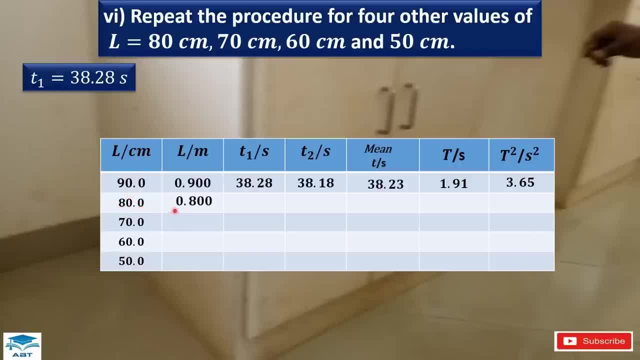 to 80 centimeters, That is 0.8 meters, But we leave it in three decimal places Because once again, we know that the time of oscillations is 60 centimeters And we can answer for system length, Assimilating time length. 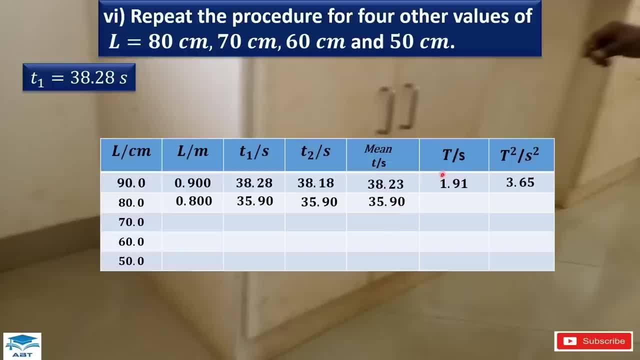 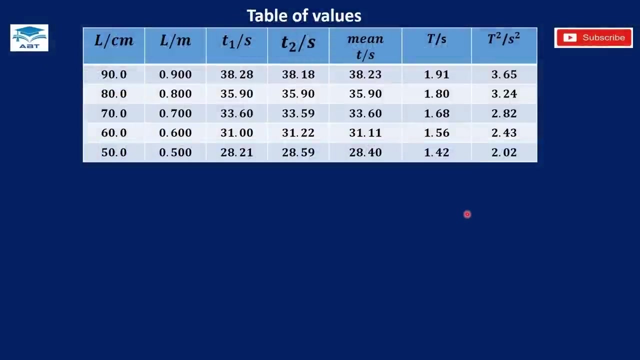 of control and control length is 150 centimeters. That is the time of oscillations- 60cm, 50cm, and tabulate the results. So this is the table of values And the numbers under each column should be in the same number of decimal. 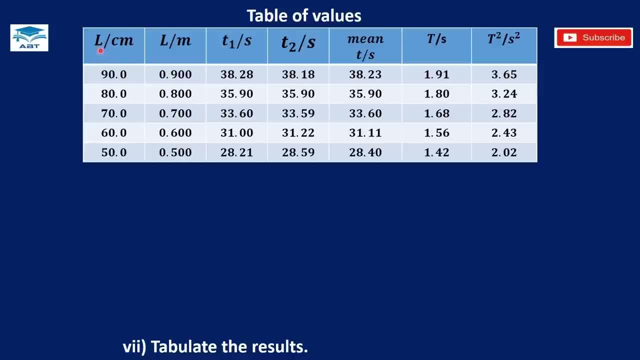 places. For instance, the length in cm, the values are in one decimal place. The values in this column, too, are in three decimal places, and all of them are in three decimal places, And the values here are in two decimal places. The values here: 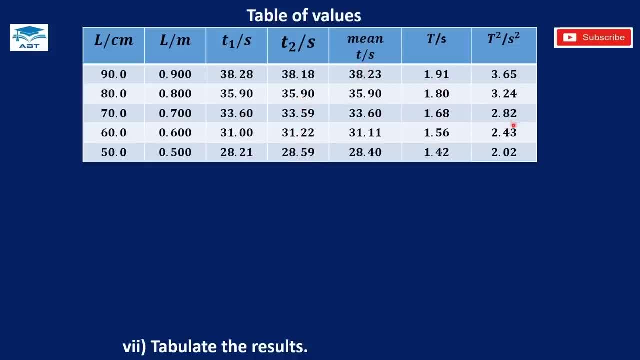 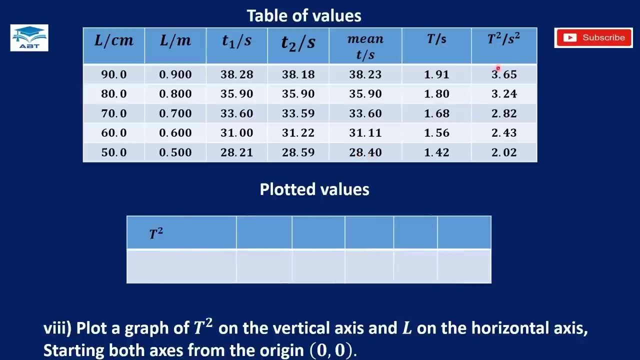 two decimal places, Two, two, two decimal places, And we are going to plot a graph of t squared on the vertical axis and L on the horizontal axis, starting both axes from the origin. So for the values of t squared we have 3.65. 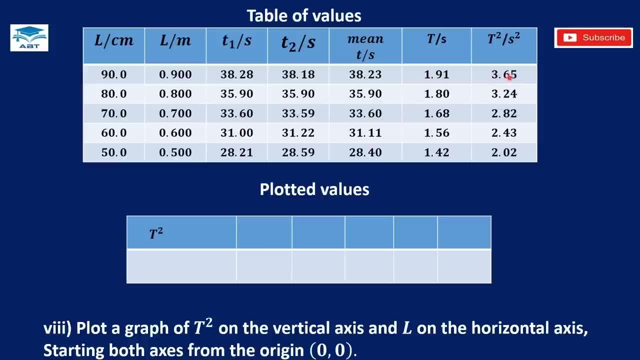 and it will be difficult to plot 3.65 on the graph. So we move this point one, two and record it as 3.65 and times 10 x-2, and the unit is second squared. So it's in standard form. 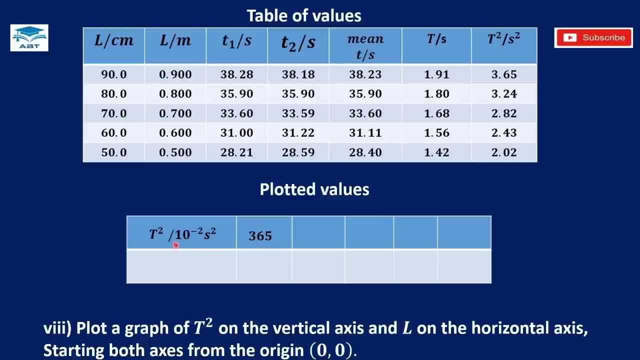 So the value 3.65 is times 10, x-2, which gives back 3.65. For the next value, we move the point one, two and we have 3,, 2, 4, the next value, 2,, 8,, 2. 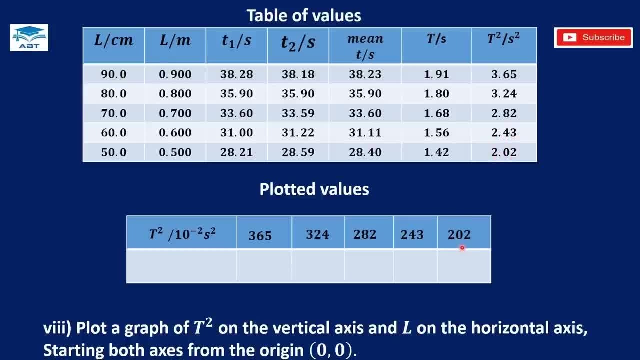 2, 4, 3 and 4: 2, 0, 2, So all the values are in standard form. That means each value is multiplied by 10 x-2 to give the value here And for the values of: 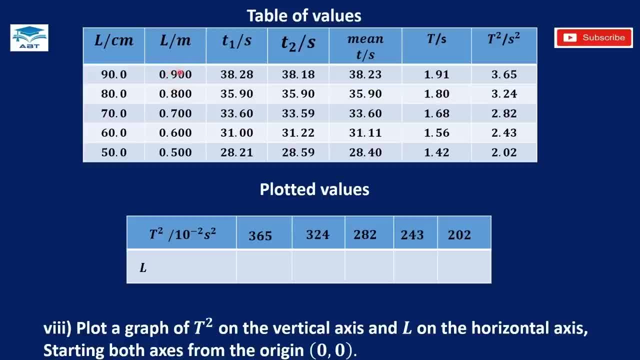 L in meters. we move the point one, two: we have 90, also times 10 x-2, and the unit is meters. The next value: we move the point one, two: we have 80, the next one is 70, 60 and 50, all times 10 x-2. 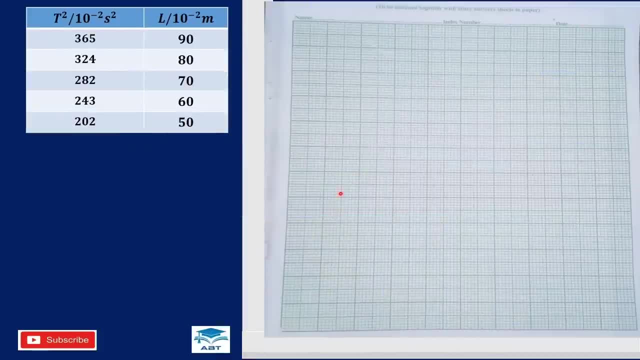 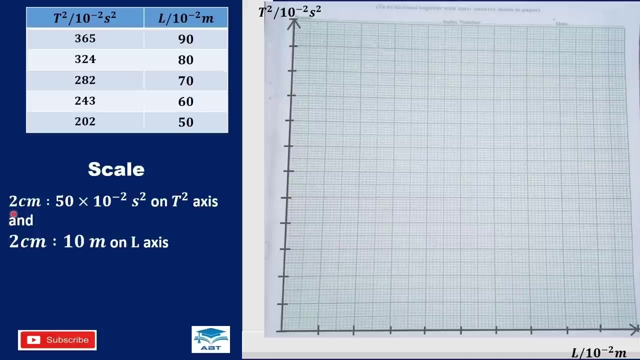 in meters. So we draw the vertical and horizontal axis. We are plotting a graph of t squared on the vertical axis and L on the horizontal axis. We choose a scale. We will choose a scale. of 2 cm is to 50 times 10 x-2. 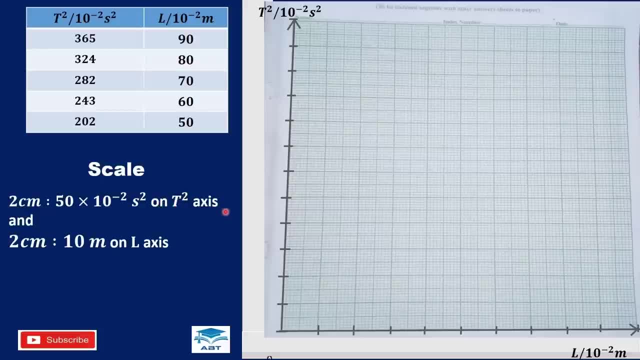 second, squared on t squared axis. So we start from 0, 50, 100, 150, 200 and so on, And on the L axis we choose a scale of 2 cm to 10 meters. So from 0 we have. 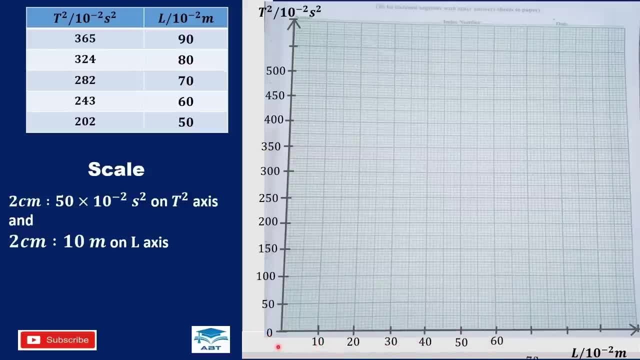 10,, 20, 30,, 40, 50 and so on. On this axis, 50 divided by 10 is 5.. So one small box on the vertical axis is 5.. And on this axis too, we have 10 divided by 10.. So one. 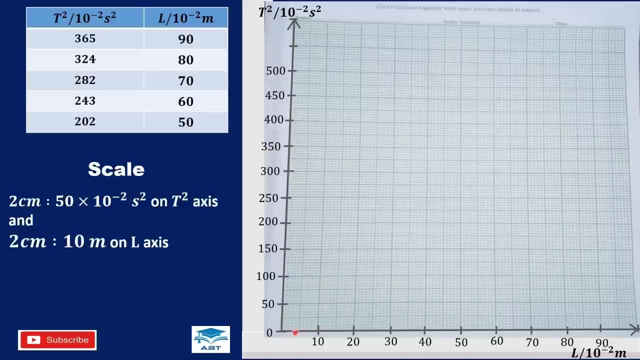 small box on the horizontal axis is 1.. Okay, so for the first point, we have 90 on the horizontal axis, 365 on the vertical axis. So we have 90 here. This is 350. One box is 5.. So 355. 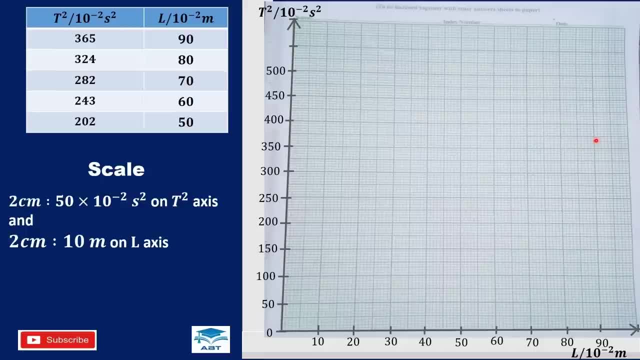 360, 365. That is 3 boxes. And the second point: we have 80 on the horizontal axis and 324 on the vertical axis, So this is 300. One box is 5.. So 300 and 5: 10. 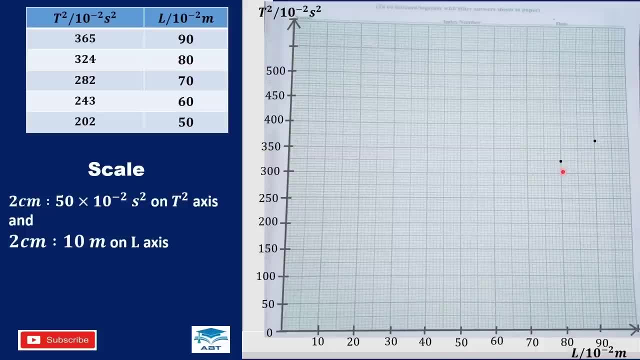 15,, 20 and the 4 will be in the next box. The next point: we have 70 on the horizontal axis, 282 on the vertical. This is 200, This is 250, So 255, 260, 65, 70. 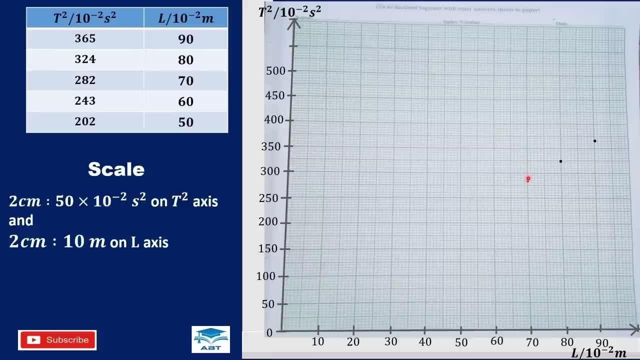 75,, 80, 82 will be in the next box. The next one is 60 and 243. This is 200. The middle will be 225, 235, 240, 243 will be in the next box, The last one. we have 50 and. 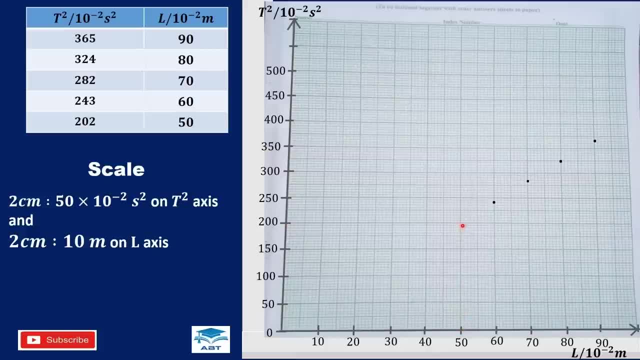 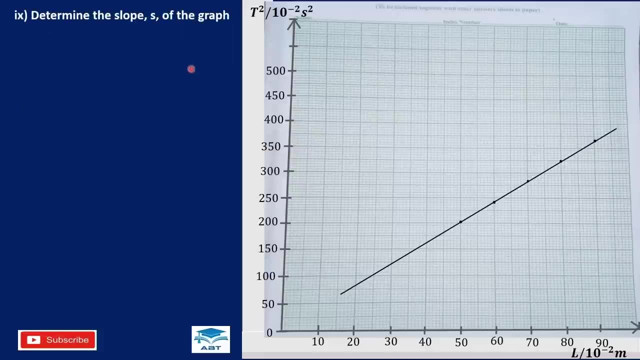 this is 200, and then 2 will enter into the next box. So we draw the line of best fit, Determine the slope S of the graph. So we draw a horizontal and a vertical line. We name here A, B and. 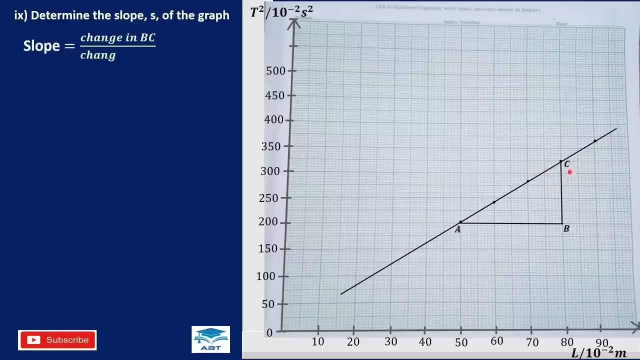 C, The slope is changing BC over changing AB. For changing BC, we have 305 and 5, 10,, 15, 20, 320 minus 200 times 10 squared negative 2, and the unit is second squared For changing AB. we have 80. 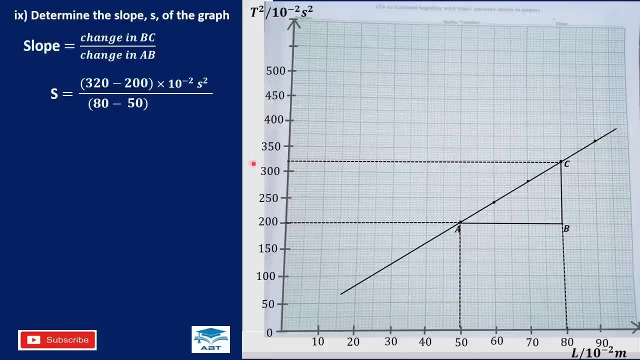 minus 50. also times 10 exponent negative 2 and the unit is meters. So times 10 exponent negative 2 will cancel out, and 320 minus 200, 120.. The unit is second squared: 80 minus 50 is 30 meters. 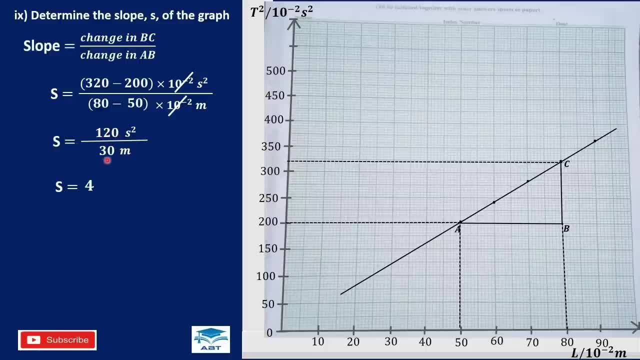 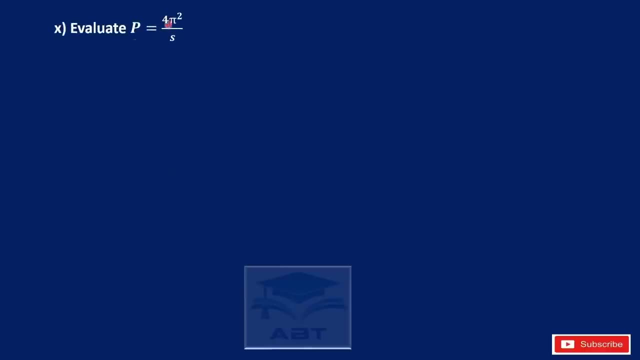 and 120 divided by 30 is 4.. At the numerator we have second squared and the reciprocal of meters is per meters. Evaluate: P is equal to 4 pi squared divided by the slope, P is equal to 3.142 and the slope is